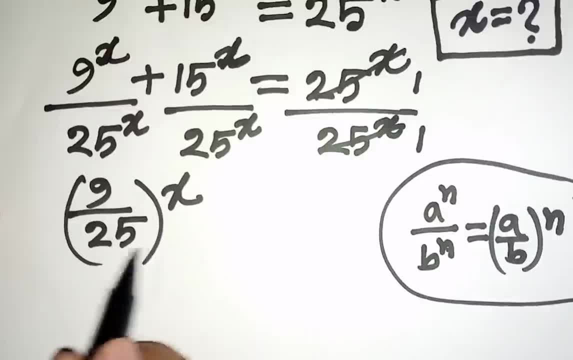 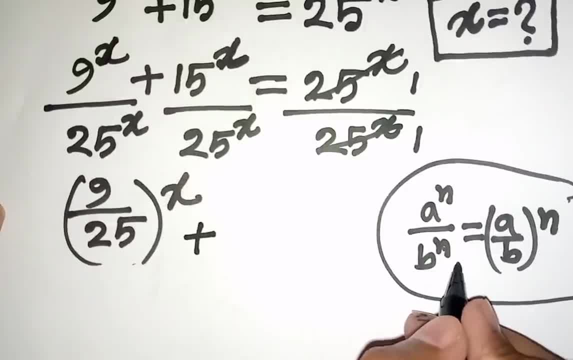 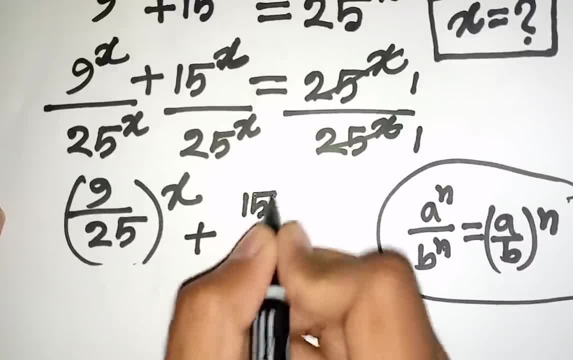 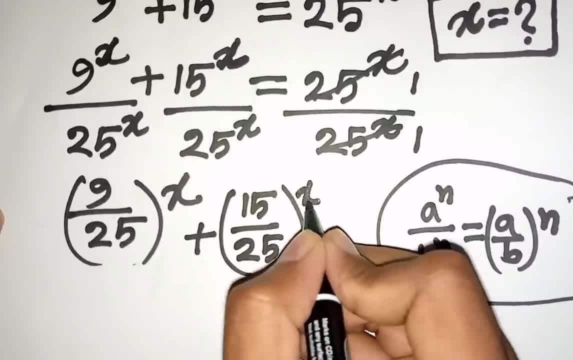 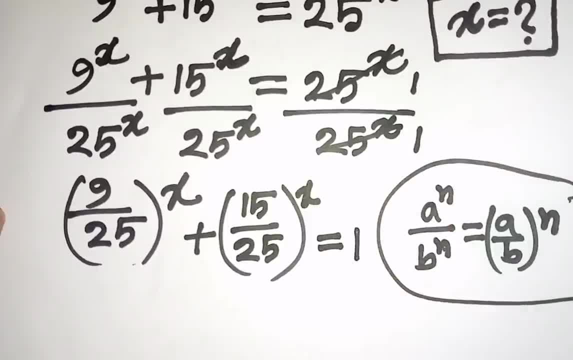 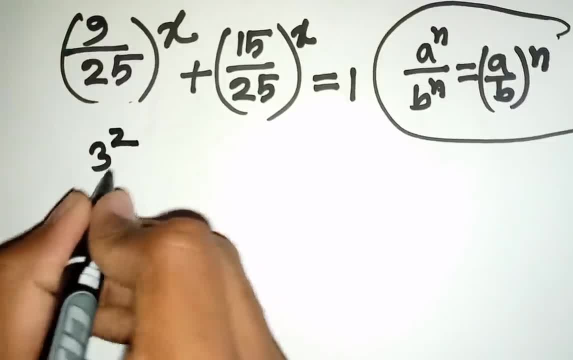 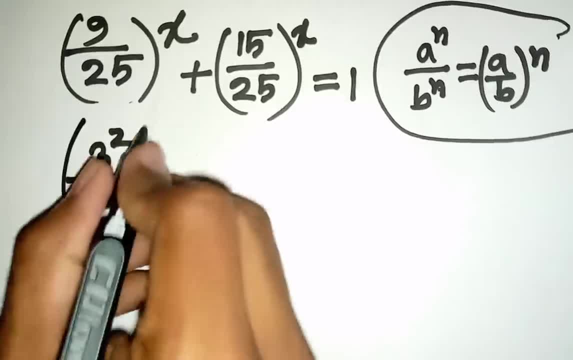 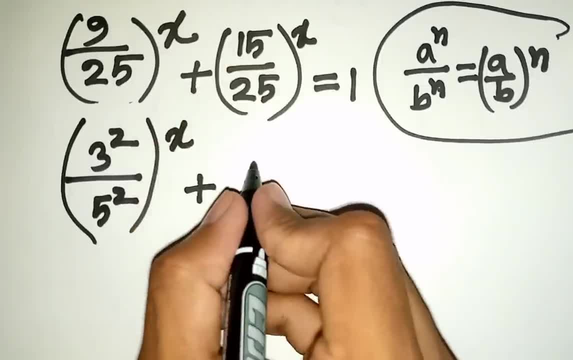 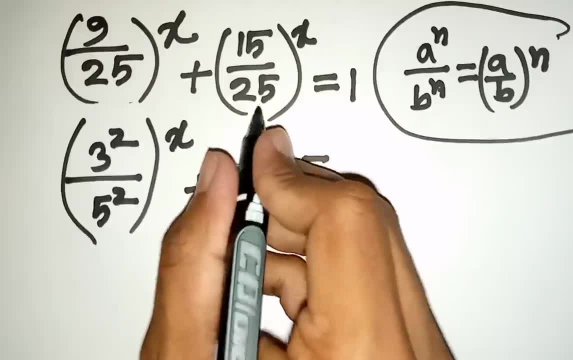 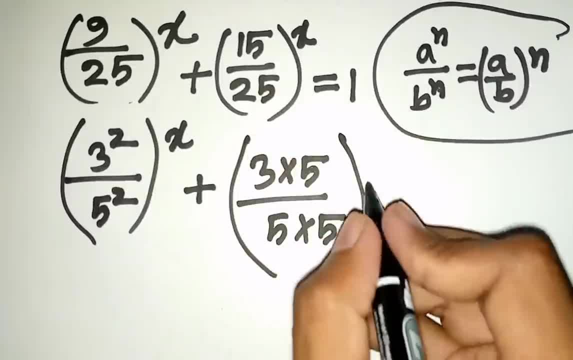 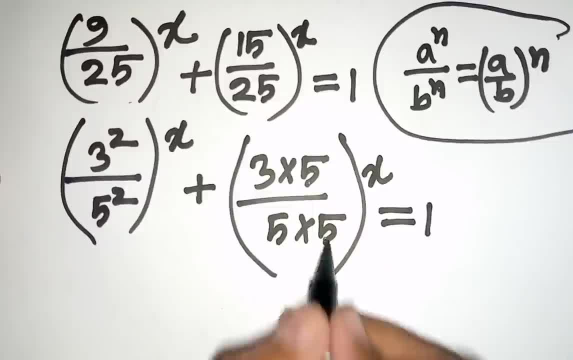 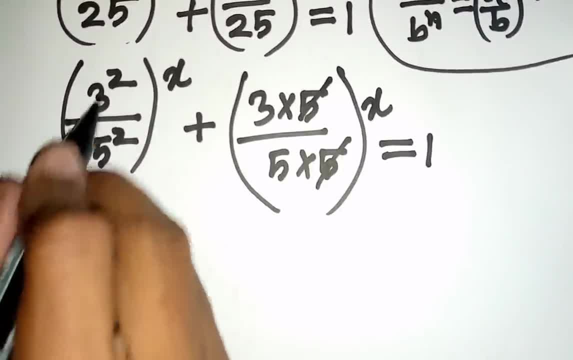 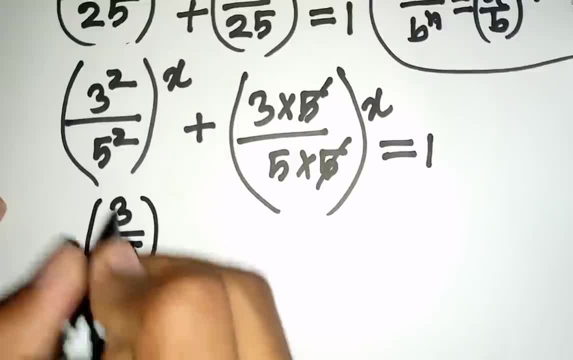 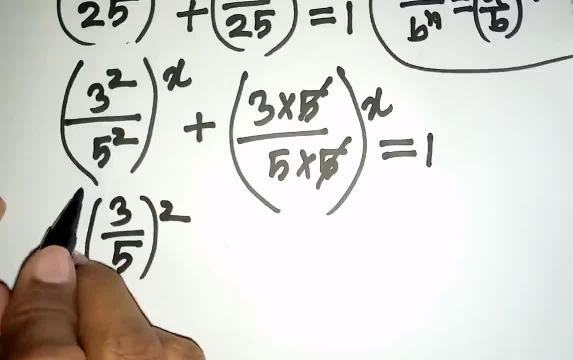 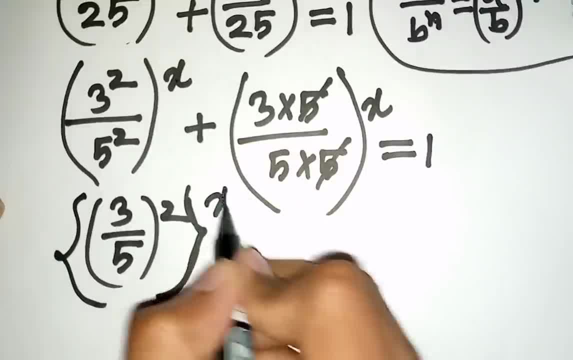 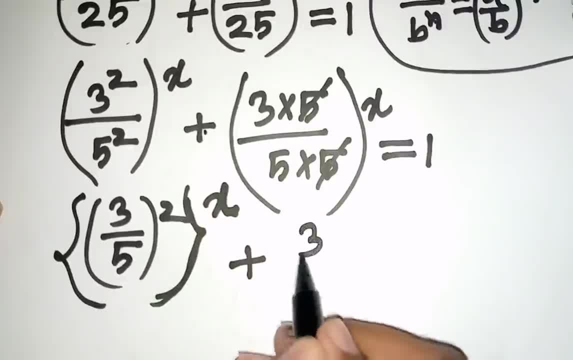 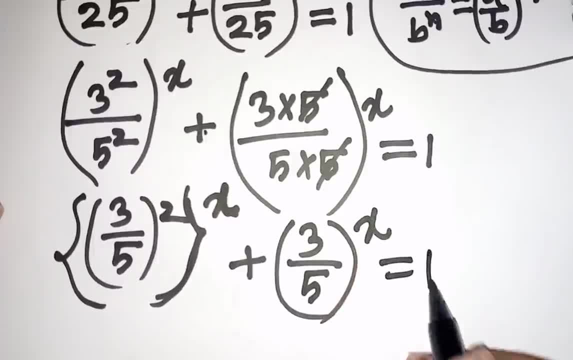 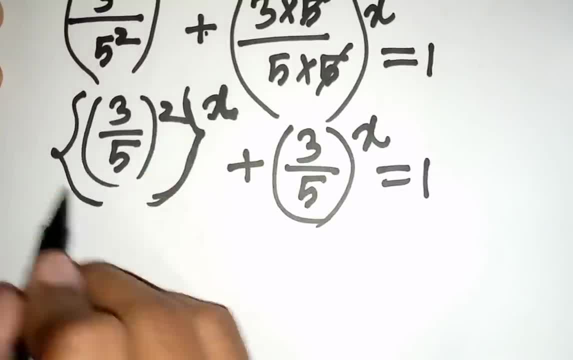 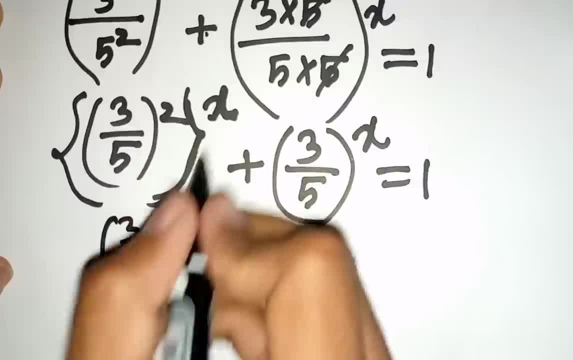 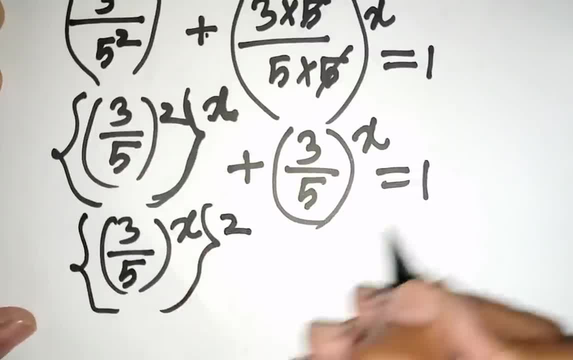 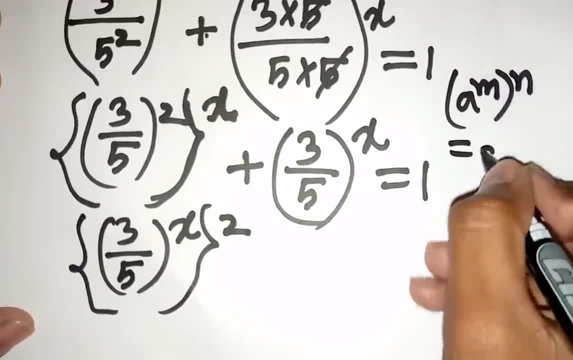 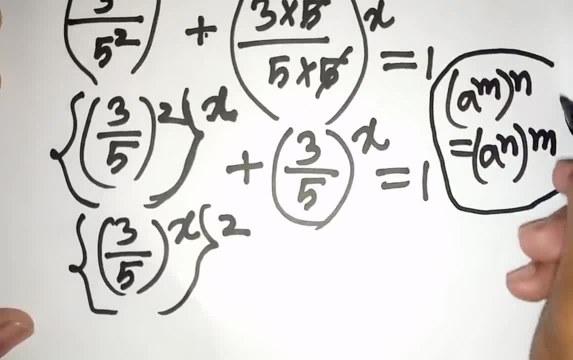 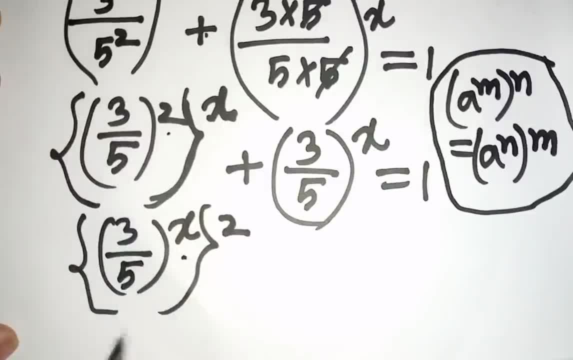 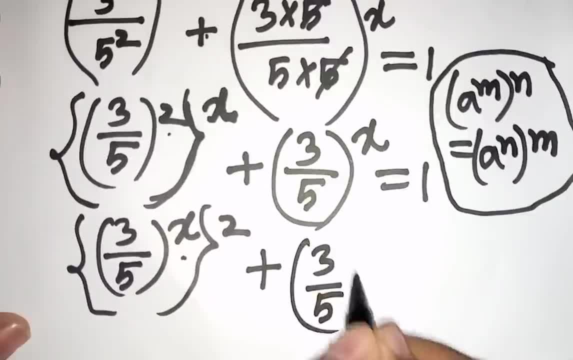 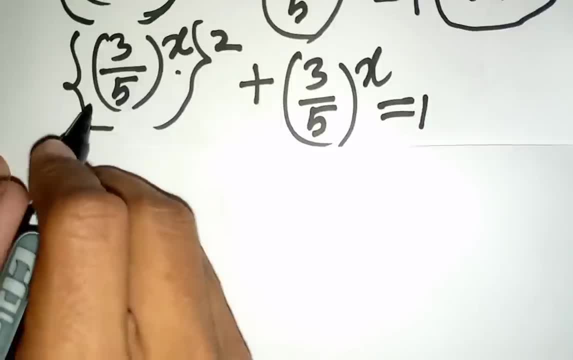 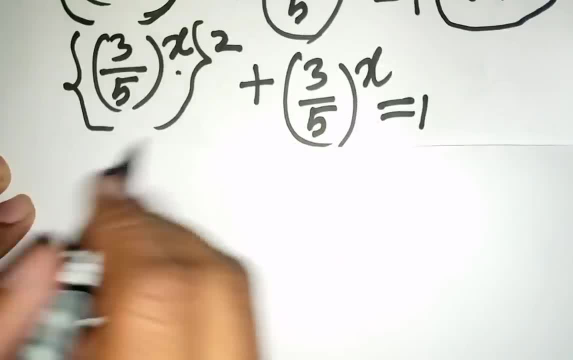 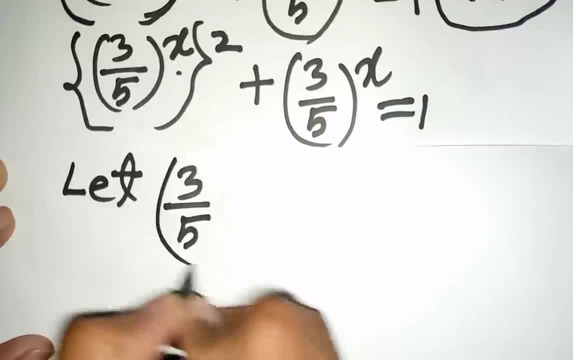 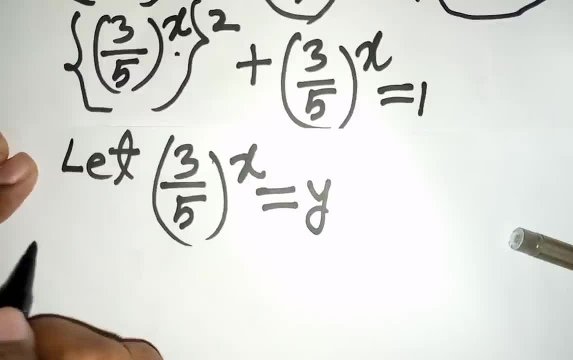 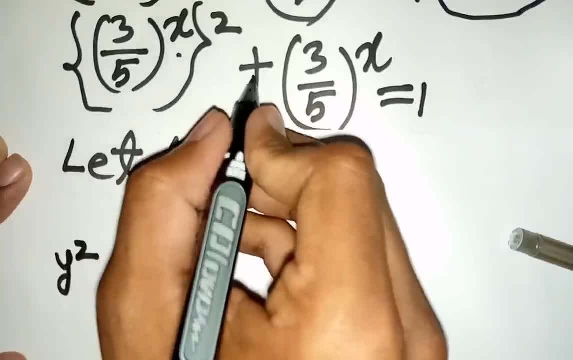 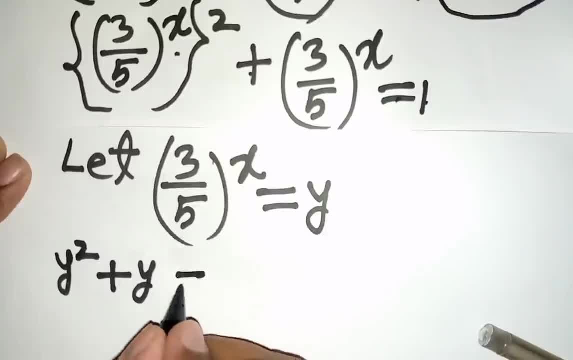 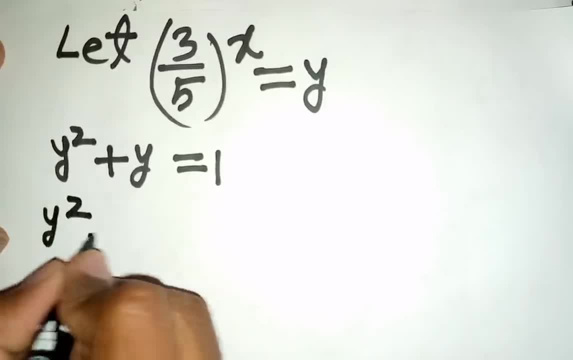 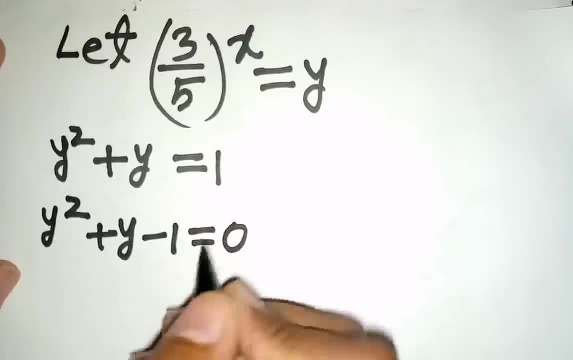 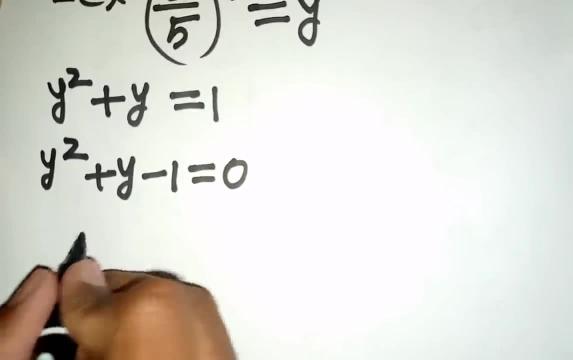 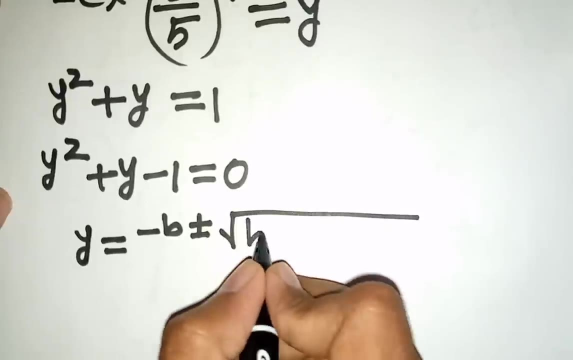 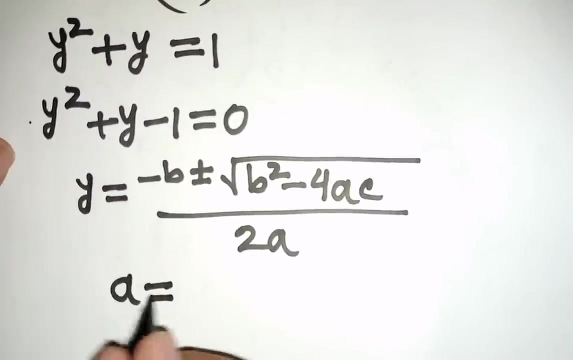 take to the left side. so this will be: minus 1 is equal to 0. now we can write here: here we can apply quadratic formula. so we can write here: y is equal to minus b, plus or minus a, square root of b square minus 4ac divided by 2a. now here a is as on, b is as on, c is as minus on. that means negative. 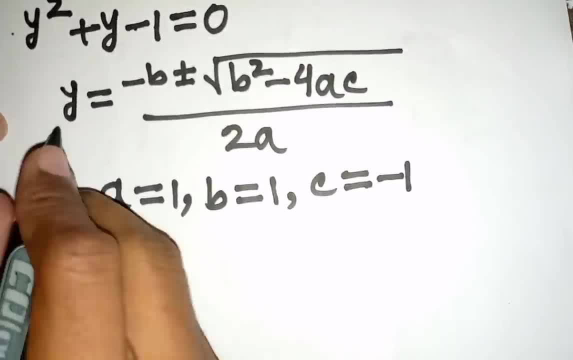 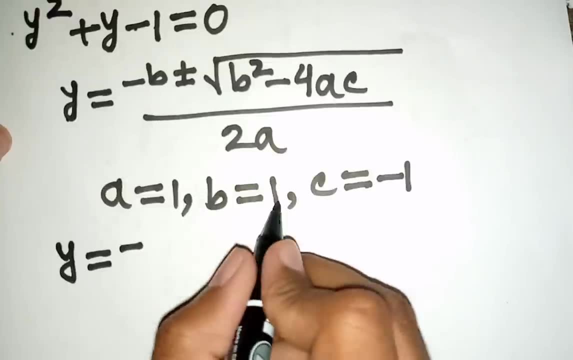 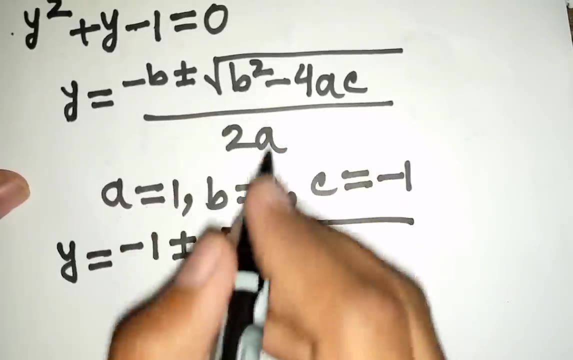 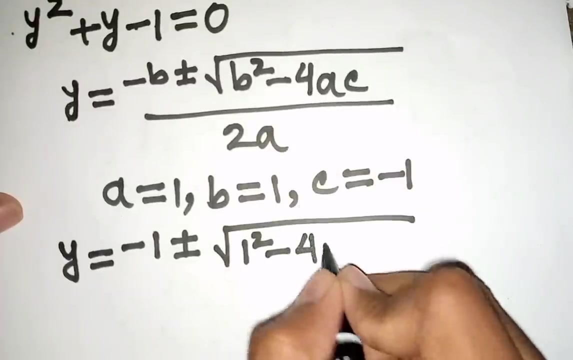 on. so we can write: here: y is equal to minus b square minus 4ac divided by 2a. now here a is as to minus b, that means 1 plus or minus a square root of b square. that means 1 square minus 4 times a. that means 1 times c, that means negative 1.. So bracket negative 1 divided by: 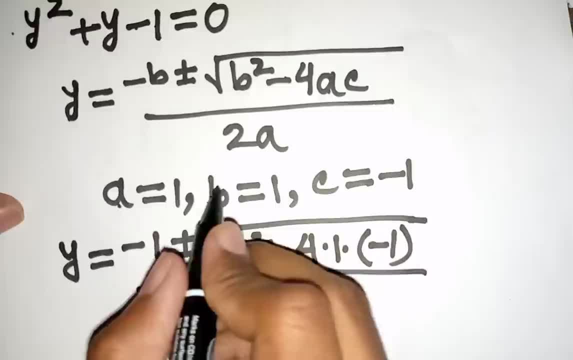 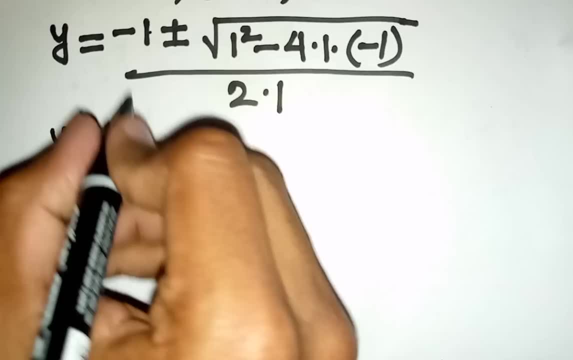 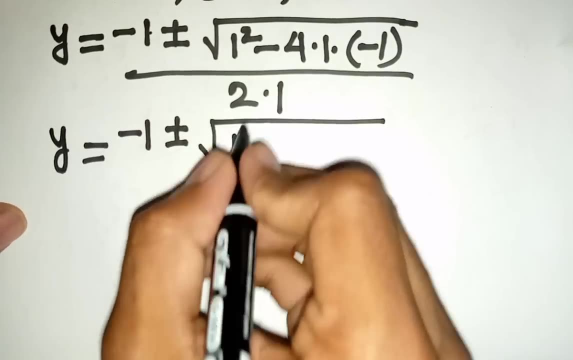 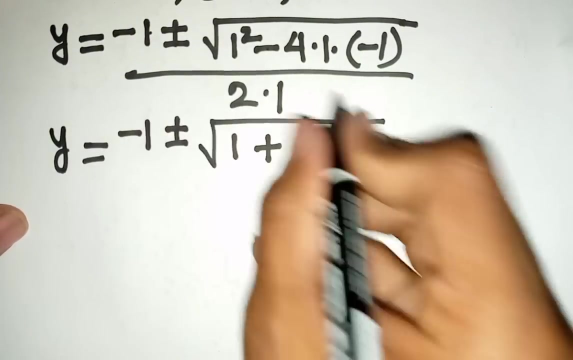 2 times a. that means 1.. Now we can write here: y is equal to minus 1, plus or minus a square root of 1 square. that means 1 minus times minus. it will be plus. 4 times 1 times 1. it will be 4 divided by 2 times 1. that means 2.. Now we can write here: 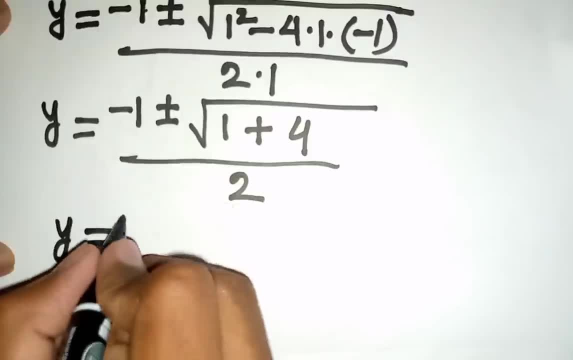 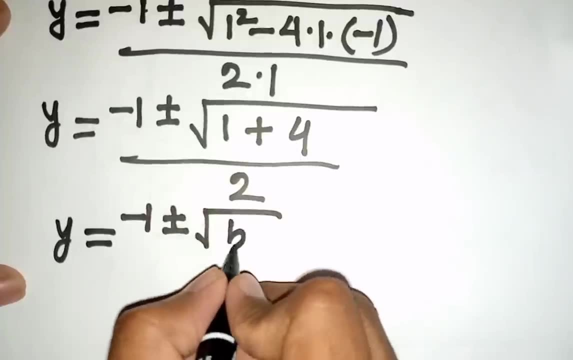 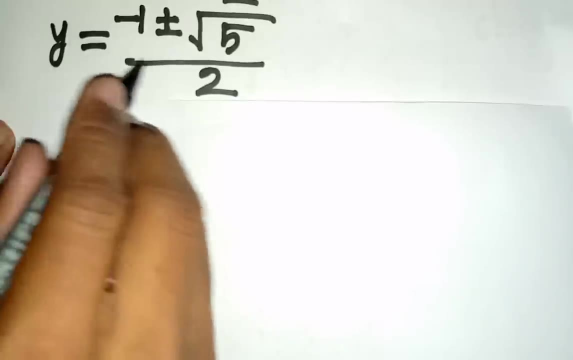 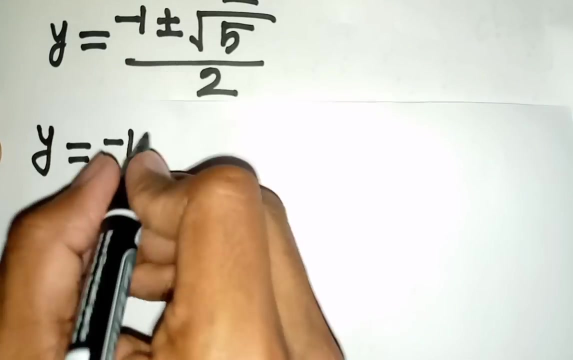 y is equal to minus 1, plus or minus a square root of 1 plus 4, that means 5 divided by 2.. Now we see here two cases, so we can write here: y is equal to minus 1 plus a square root of 5. 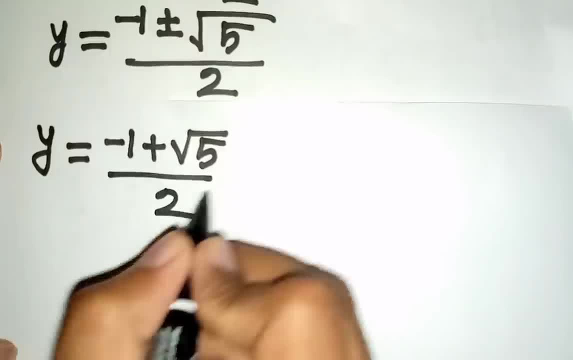 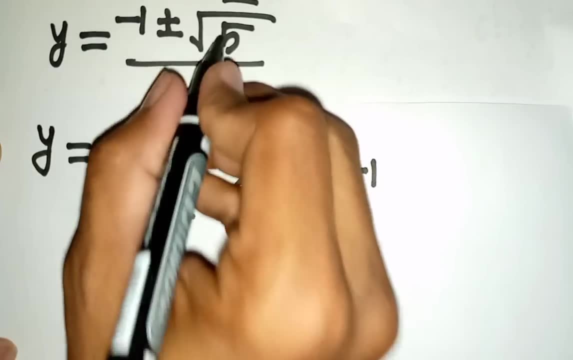 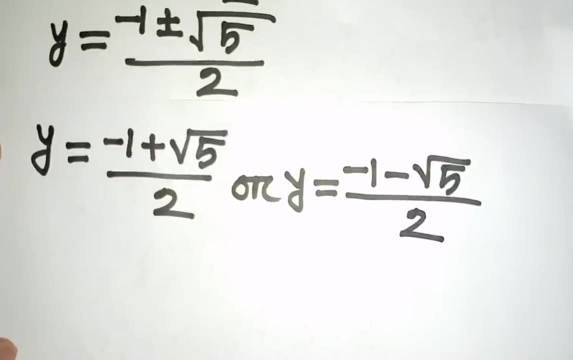 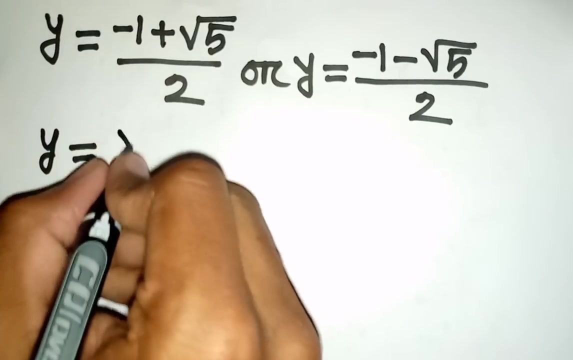 divided by 2, or y is equal to minus 1 minus a square root of 5 divided by 2.. Now we can write here: y is equal to. Y is equal to minus 1 plus a square root of 5. that means square root of 5 minus on divided by 2. 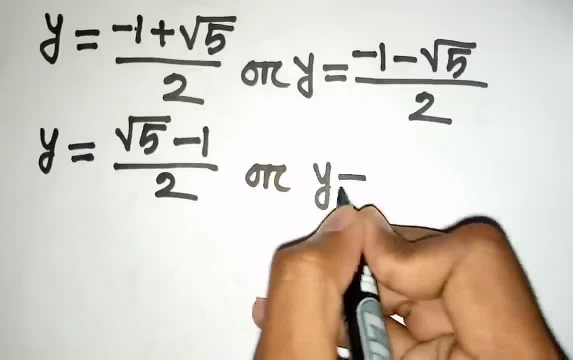 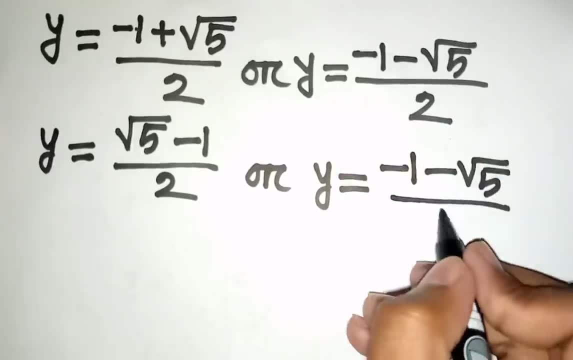 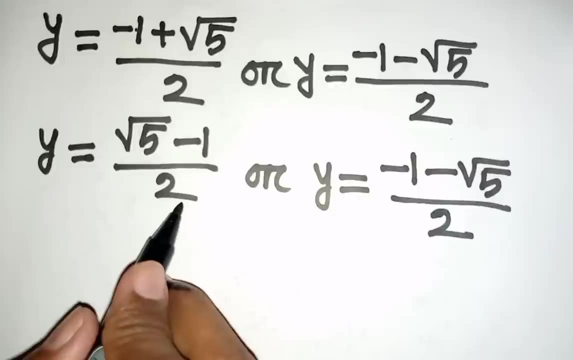 or y is equal to minus on minus a square root of 5 divided by 2.. Now, y is equal to a square root of 5 minus 1 divided by 2. but remember y that means- let theta server say that- a need to be. 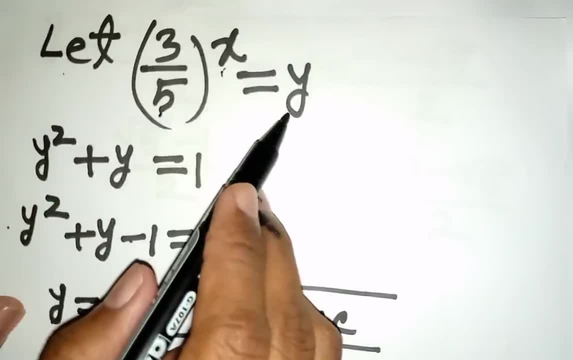 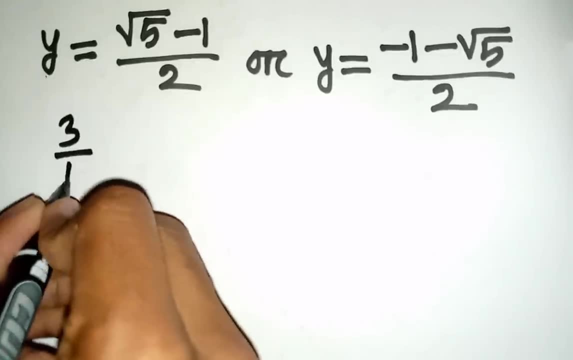 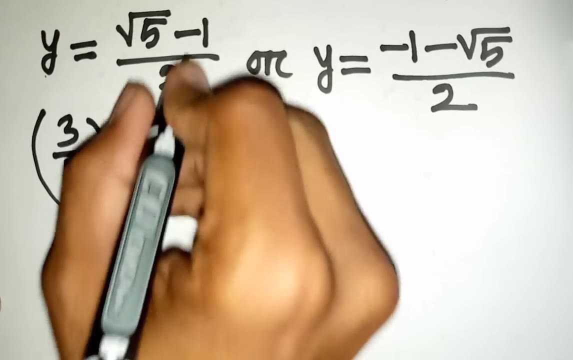 3 divided by 5. bracket power x is substituted by y, so y that means 3 by 5, bracket power x, so y that means 3 by 5. bracket power x is equal to square root of 5 minus 1 divided by 2, or. 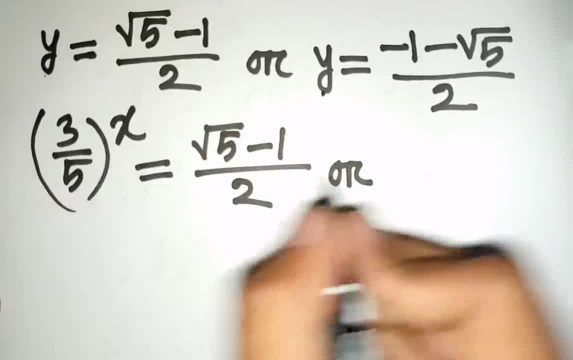 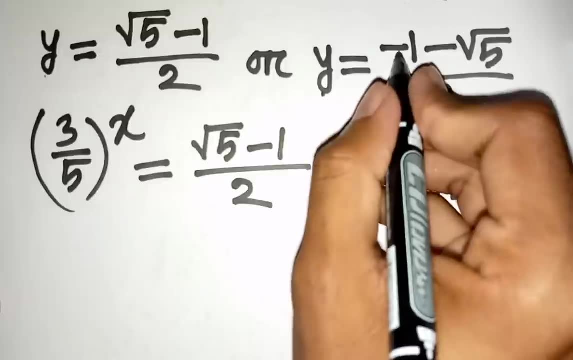 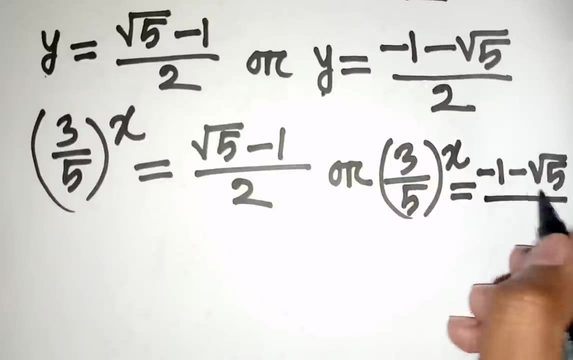 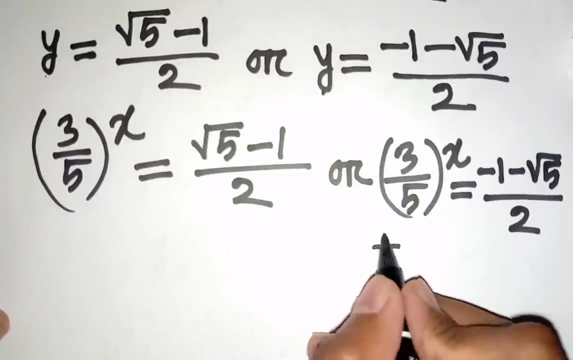 y. that means 3 by 5 bracket power x. 3 by 5 bracket power x is equal to minus 1, minus square root of 5 divided by 2. now we see 3 by 5 bracket power. any number is always positive, but minus 1, minus square. 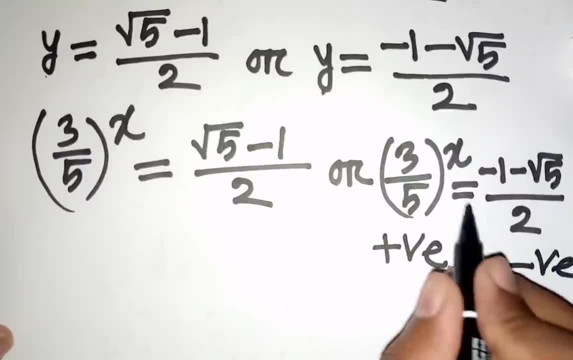 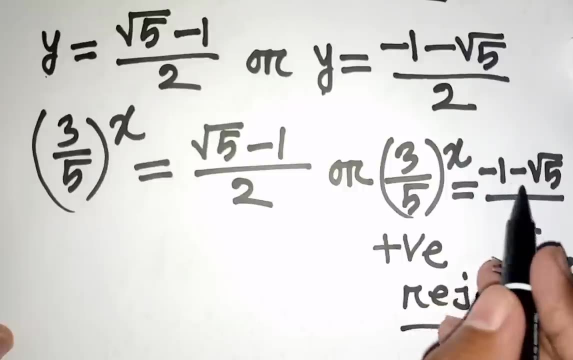 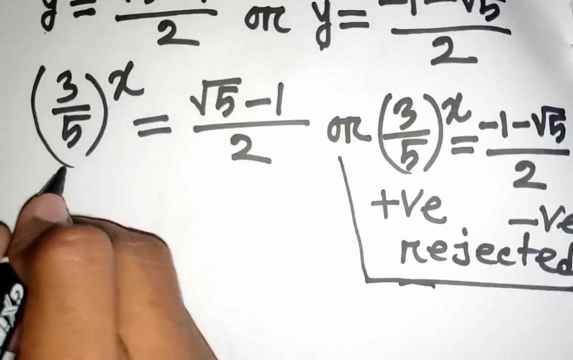 root of 5 divided by 2.. This is negative. so positive is not equal to negative. so this is rejected. because 3 by 5 bracket power, any number is greater than 0, but minus 1, minus square root of 5 divided by 2, is less than 0. so this is rejected. Now here we take log both sides so we can write here. 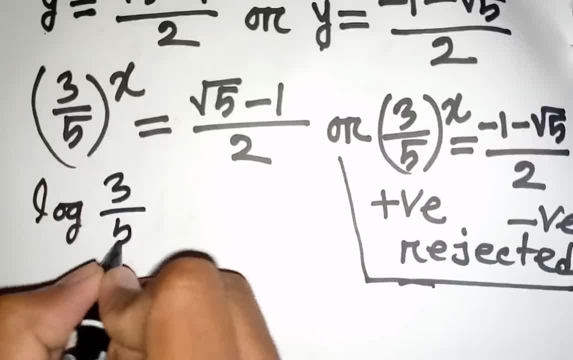 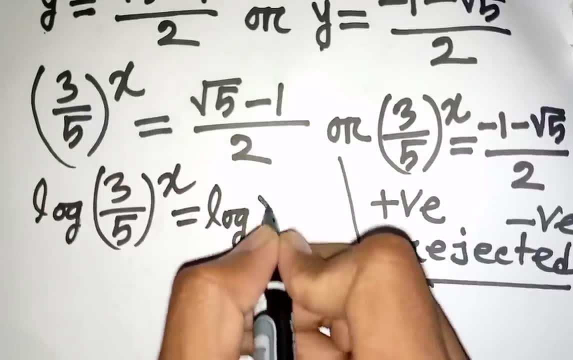 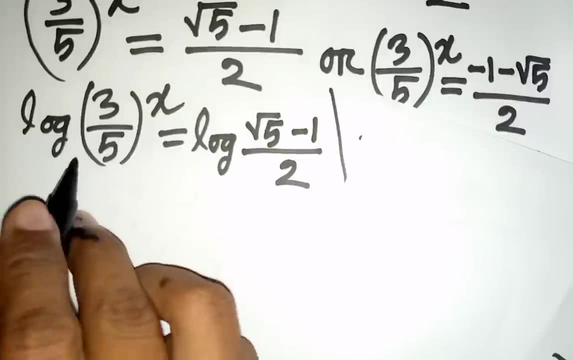 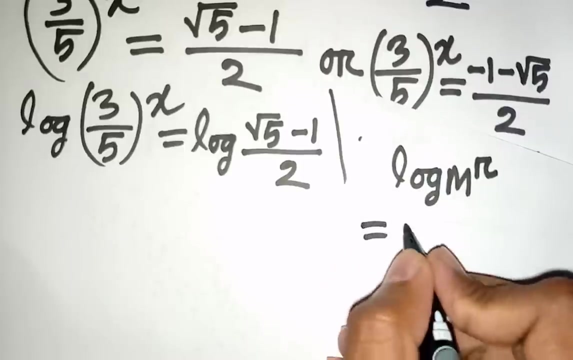 log of 3 by 5. bracket power x is equal to log of square root of 5 minus 1 divided by 2.. Now here we can apply this formula: log m power r is equal to r log m. that means this power move to here, so according. 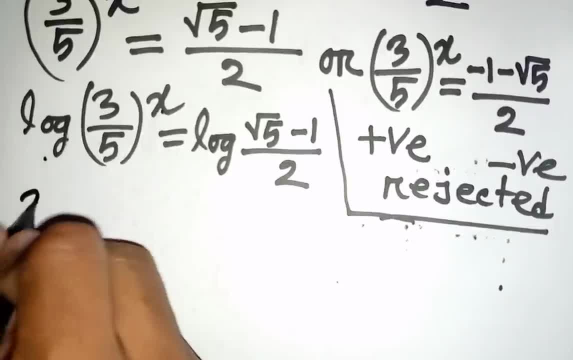 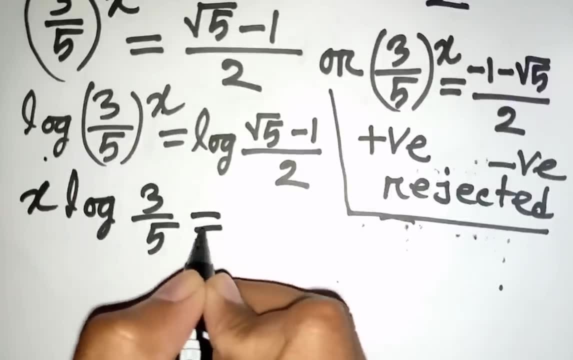 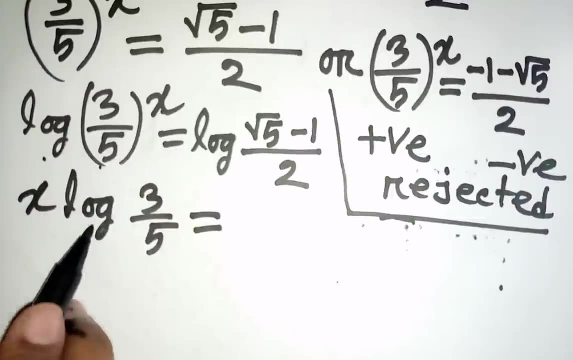 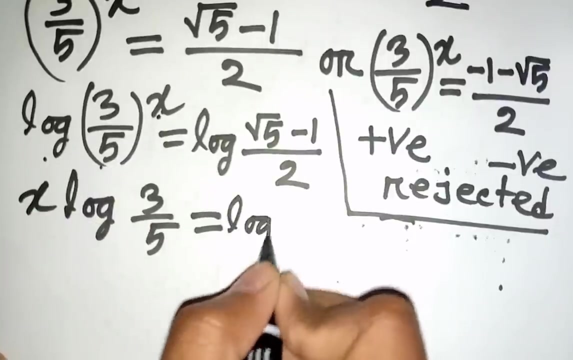 to this formula we can write here: x log 3 by 5 is equal to: so log 3 by 5. bracket power x is same as x log 3 by 5. this power move to here now is equal to log a square root of 5 minus 1. 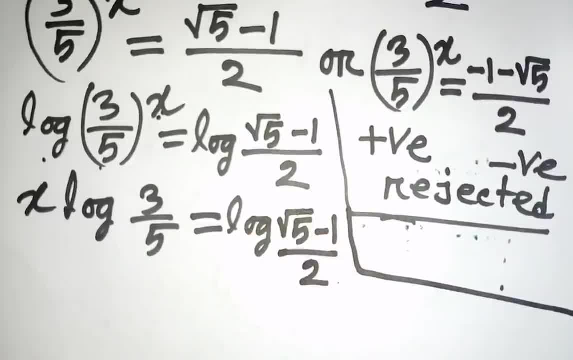 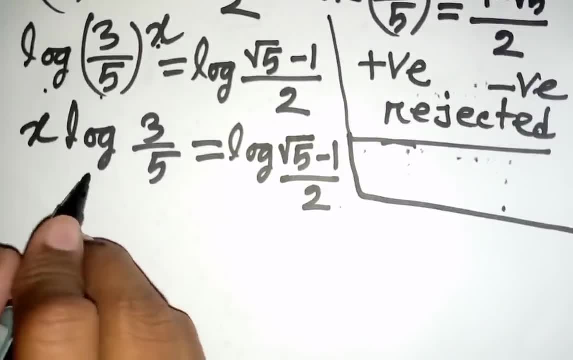 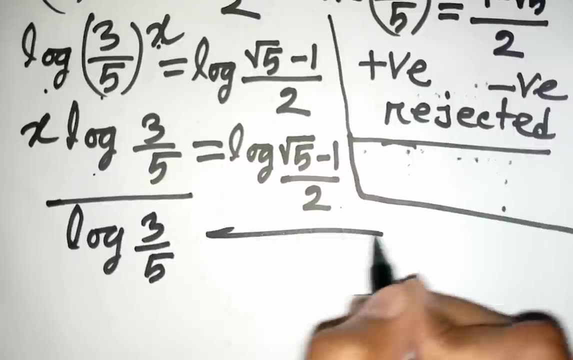 divided by 2.. 2- now we can write here. we see we need the value of X. so we divided by log 3 by 5, both sides. so divided by log 3 by 5, divided by log 3 by 5, now this log 3 by: 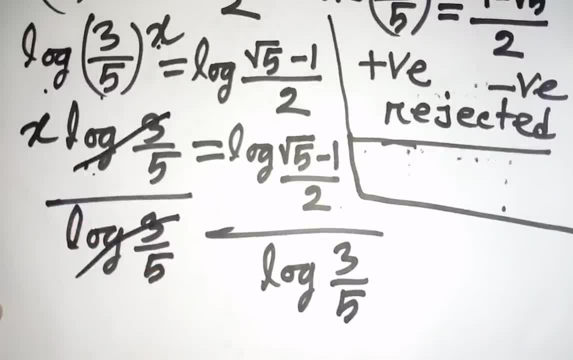 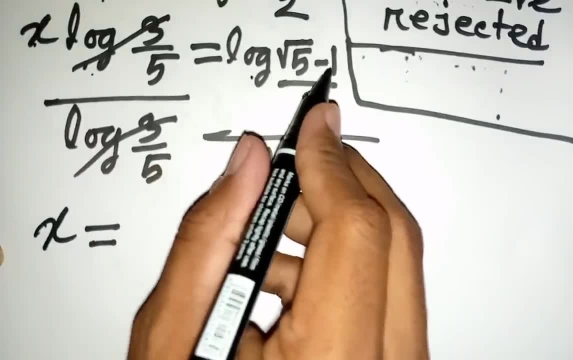 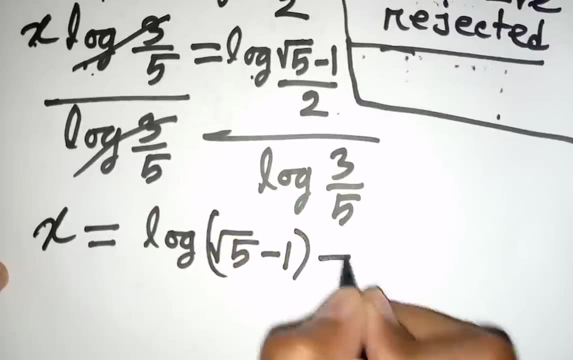 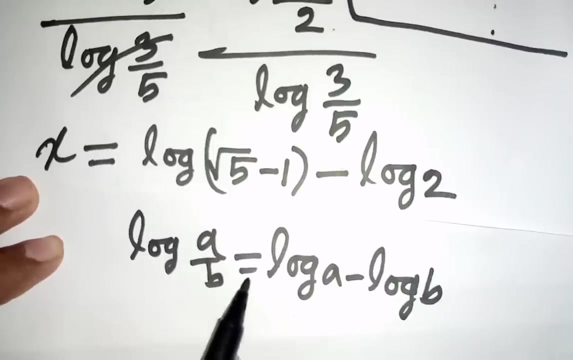 5. this log 3 by 5 will be cancelled. so here X is equal to log S square root of 5 minus 1 divided by 2 is same as log S square root of 5 minus 1 minus log 2. according to this formula, log a by B is equal to log a minus log B now divided. 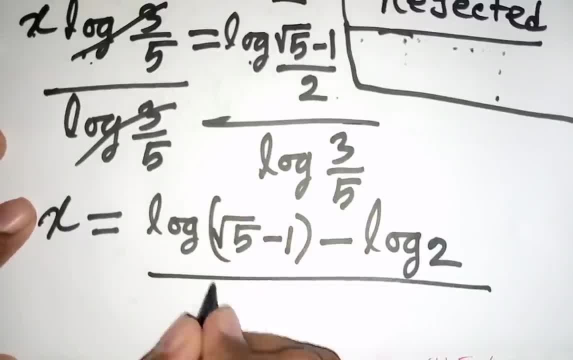 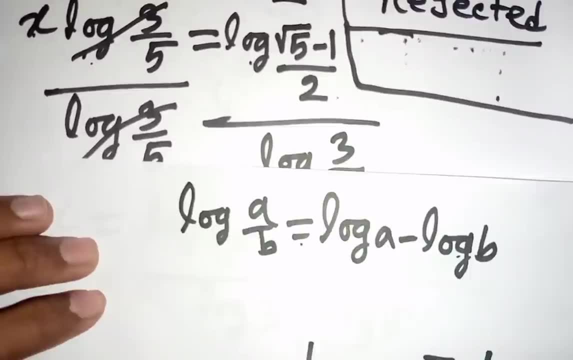 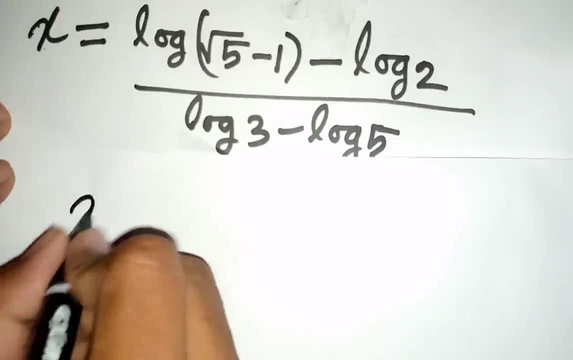 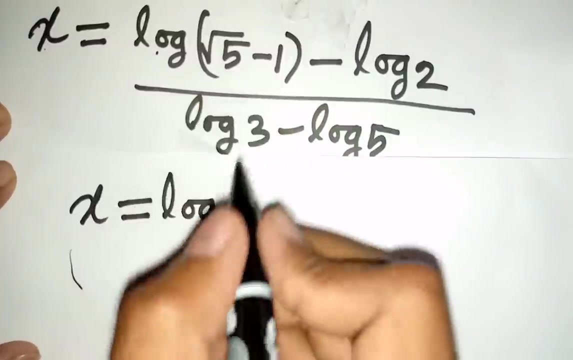 by log 3 by 5 is same as log 3 minus log 5. according to this formula, log a by b is equal to log a minus log b. Now we can write here: x is equal to log bracket square root of 5. that means 2.236. 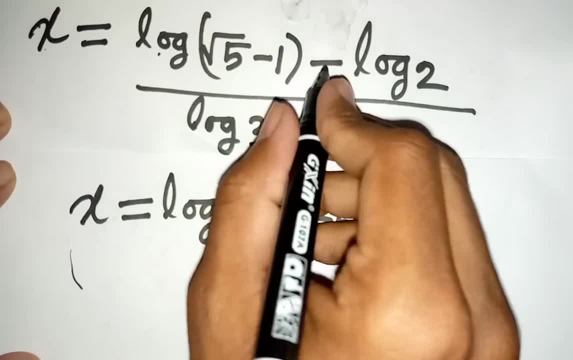 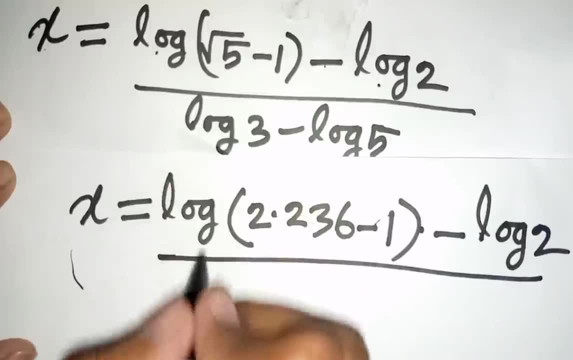 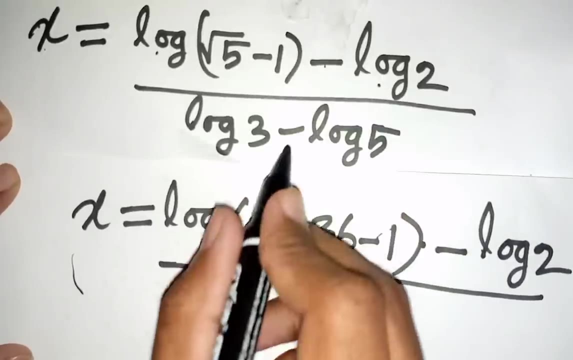 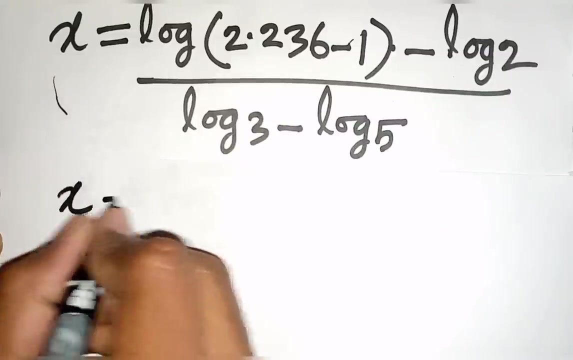 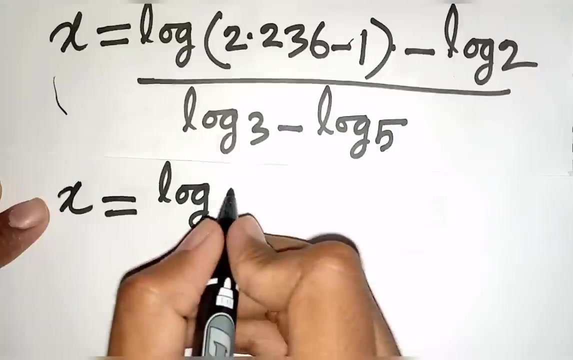 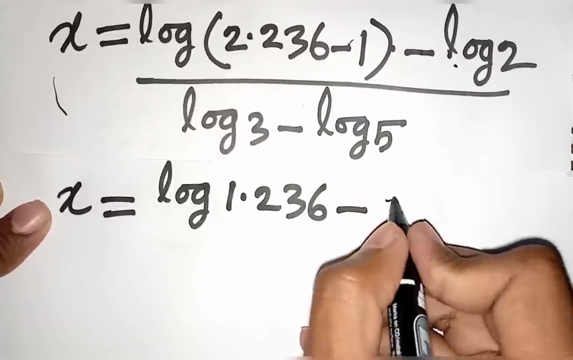 minus 1, minus log 2, divided by log 3, minus log 5, minus log 5.. Now we can write here: x is equal to log 2.236.. minus 1, it will be 1.236 minus. the approximate value of log 2 is 0.3 divided by the approximate.